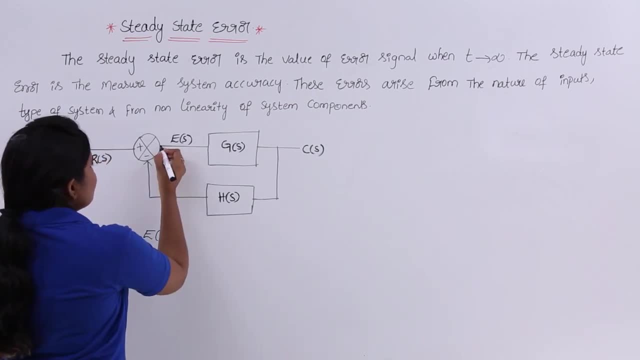 into E of S is equal into. So the combination of R of S and this feedback signal. Feedback signal is nothing but C of S into H of S. So here our feedback signal is C of S into H of S, where E of S is equivalent to combination. 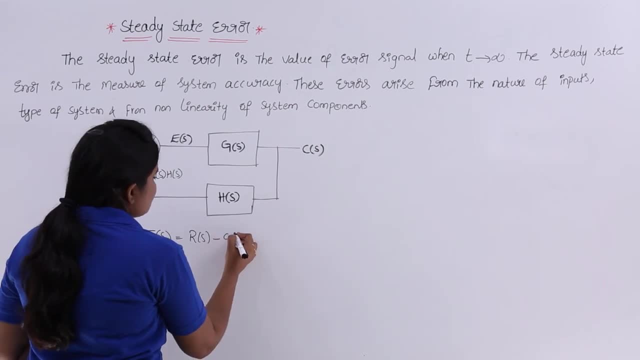 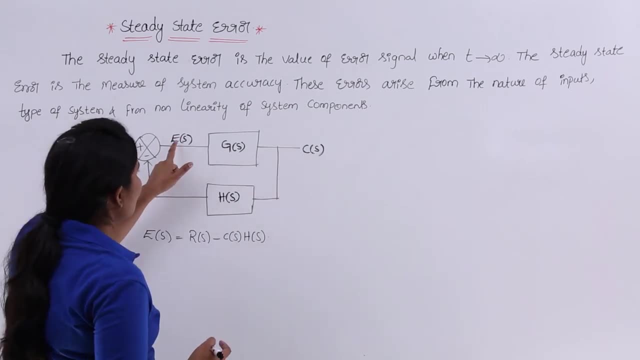 of these two. that means R of S minus C of S into H of S. You can see, C of S is the combination of E of S into G of S. So since C of S is equivalent to E of S into G of S, I am going. 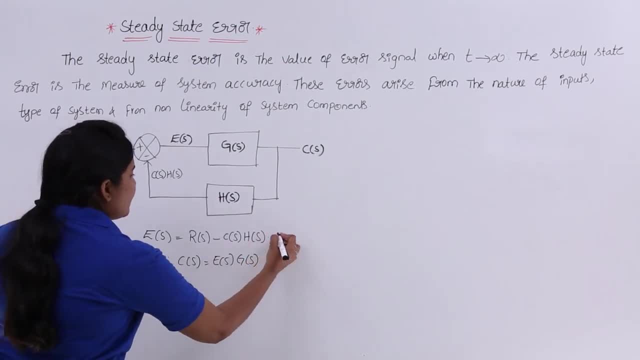 to substitute the same error. So this is the same in this equation. Then my equation 1 is going to modify like this: E of S is equivalent to R of S minus in place of C of S. I am going to write E of S into. 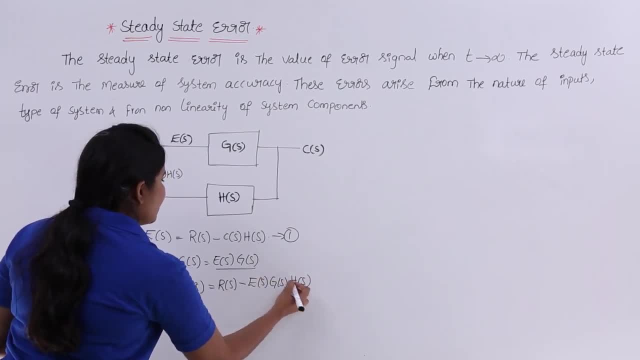 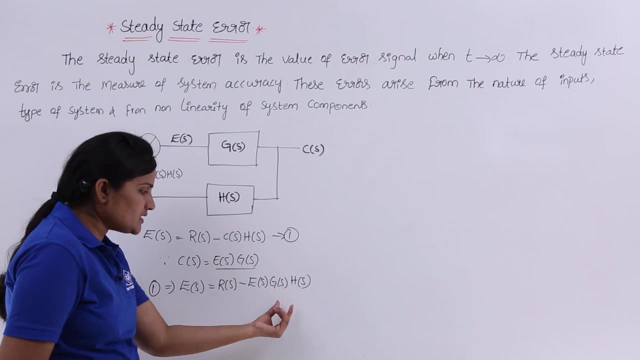 G of S into H of S. So in place of C of S, I replaced E of S into G of S, So as this side I am having E of S, here also E of S, I am sending this E of S term to this side and 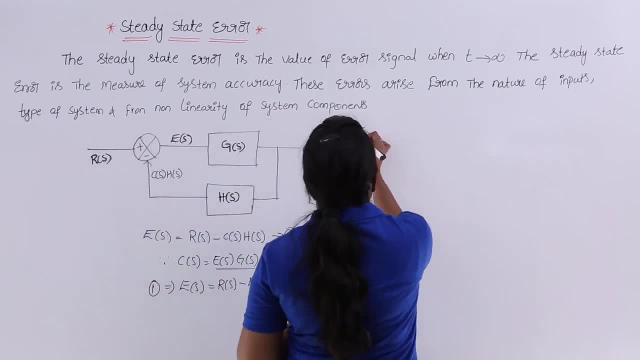 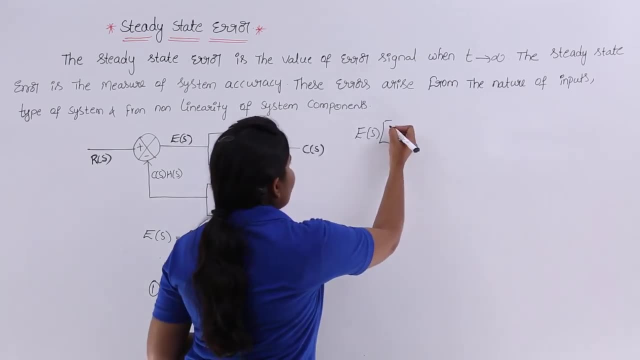 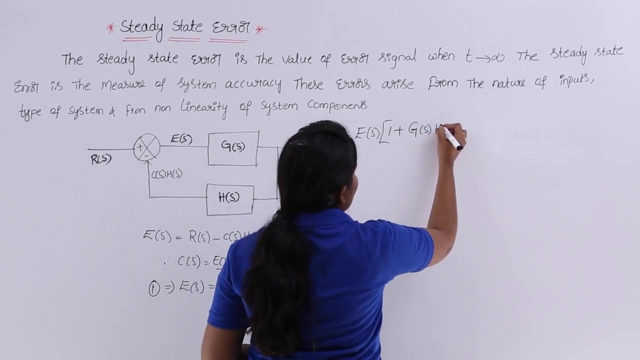 I want to take common of that E of S. So now, E of S into when I send this side, this term, when I send this side. So I am going to get E of S into one place. So remaining is G of S into H of S. G of S into H of S is: 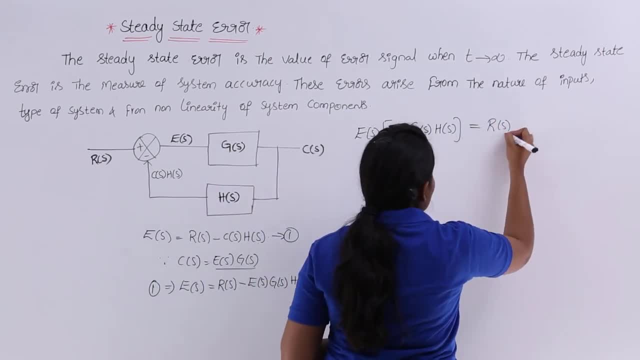 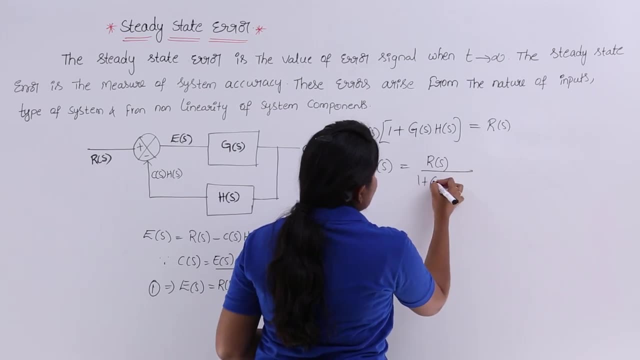 equivalent to remaining is R of S. that means input signal, If you want this error signal. so E of S is equivalent to R of S by 1 place G of S into H of S. So this is E of S into H of S. 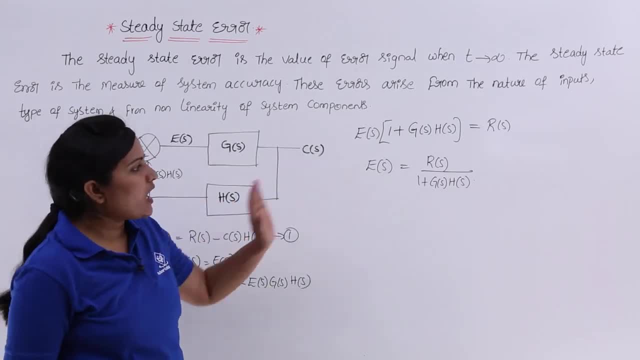 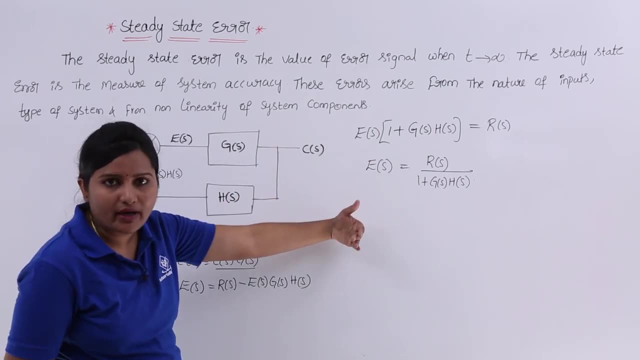 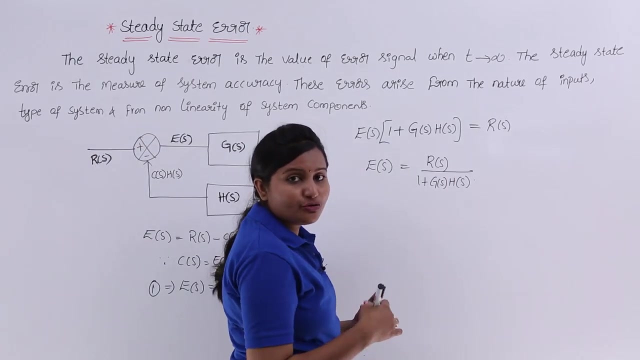 So then how we will get E of T. so that means this is error signal, but in frequency domain. If you want time domain of this error signal, then as this is in Laplace transform, we need to consider inverse Laplace transform to get time domain of this error signal. that means: 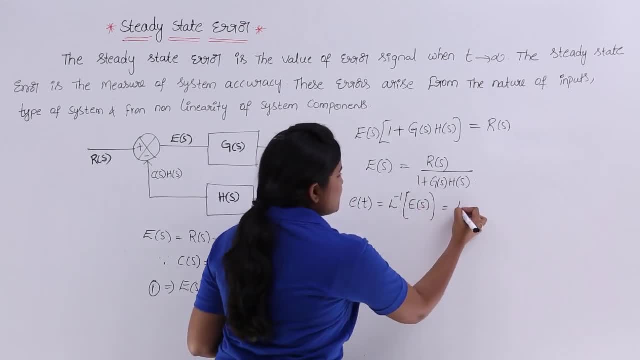 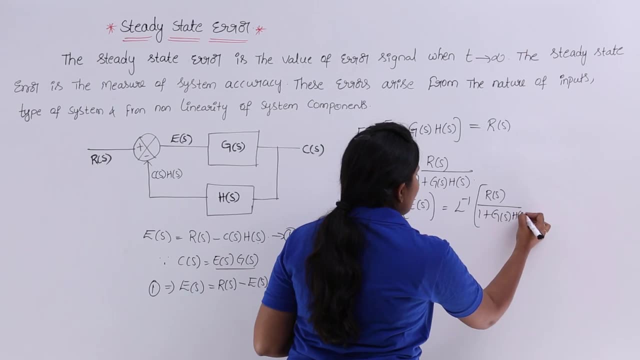 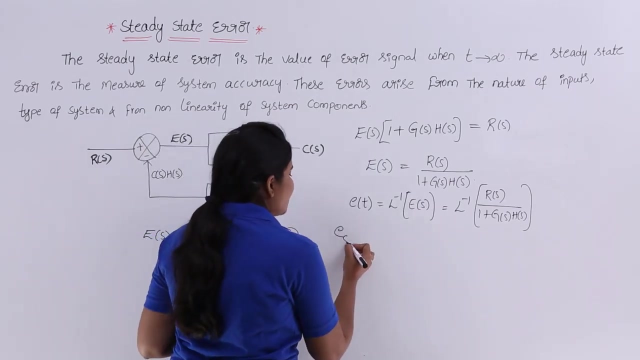 inverse Laplace transform of E of S. So that means inverse Laplace transform of R of E of S divided by 1 plus G of S into H of S will give you the error signal. Then what is meant by a study state error? Study state error, so the study state error. 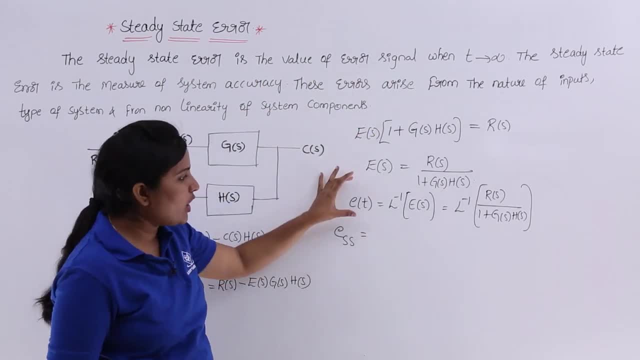 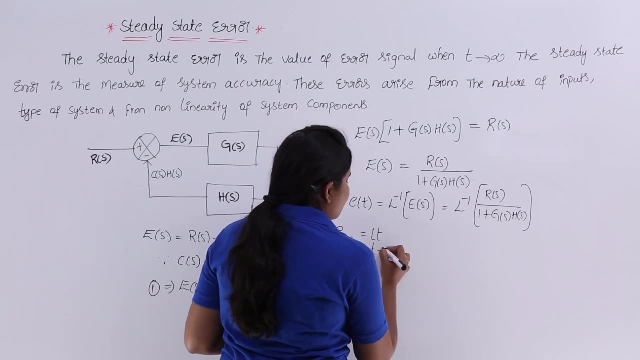 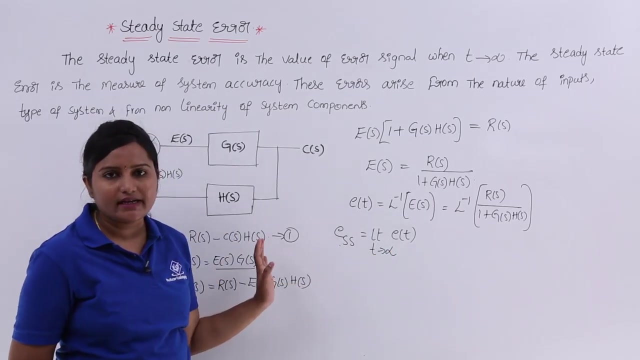 is the value of error signal. when t tending to infinity, we got the error signal. So study state error is the value of error signal at t tending infinity. So limit t tending to infinity. E of t is nothing but study state error According to the definition. if you got error, 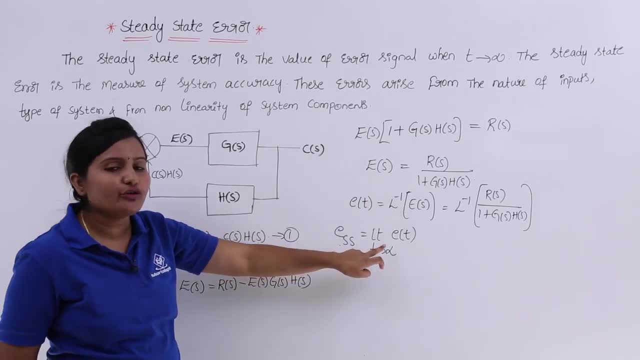 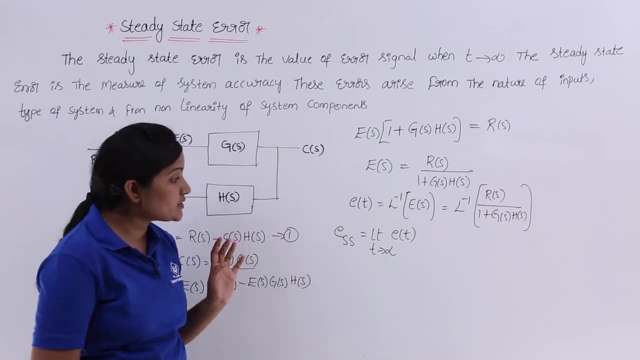 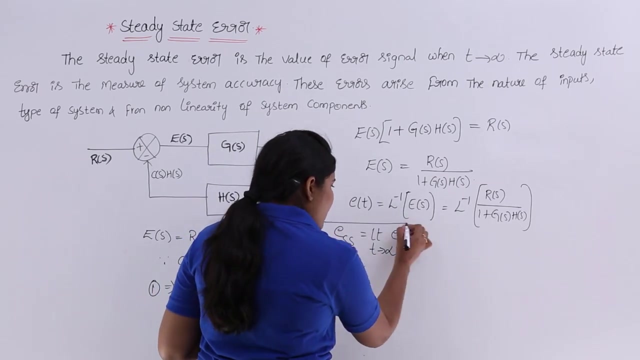 signal. the value of this error signal at t tending to infinity will be study state error. S. S represents study state, E represent error, study state error. this is very important formula. Now I applied this t tending to infinity, So this is equivalent to: this is one of the 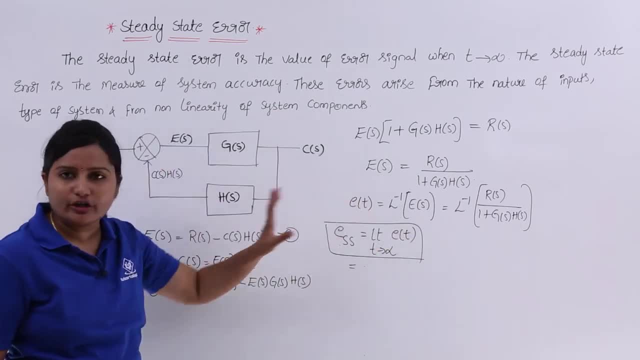 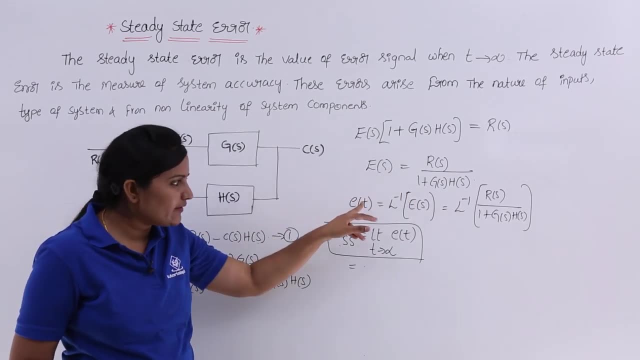 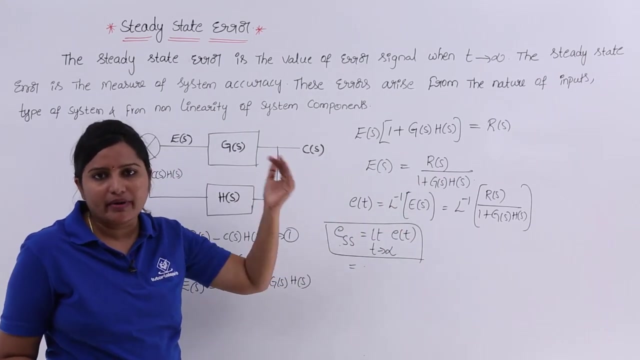 formula you need to keep in mind in some problems we are going to use this formula, or you can apply this formula or, if you felt, if they given E of S, they did not given E of t, if they given E of S, to apply this formula again, you need to consider inverse Laplace transform. 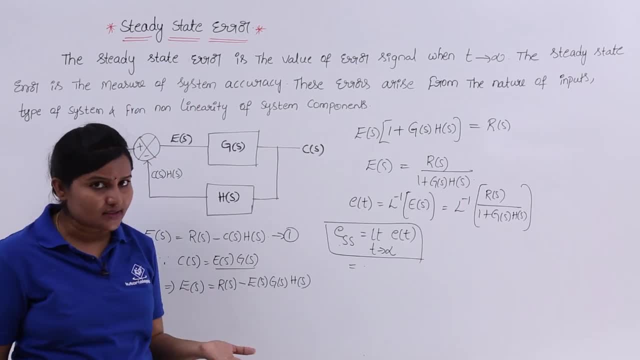 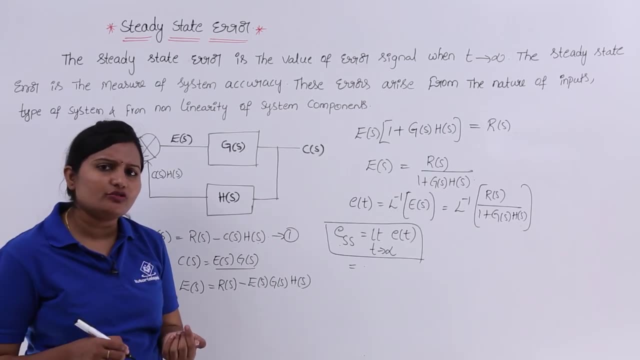 and after that you need to substitute t tending to infinity and all this. So I am going to use final value theorem here. we already discussed at this final value theorem and initial value theorem in Laplace transform in signals and systems topic also. 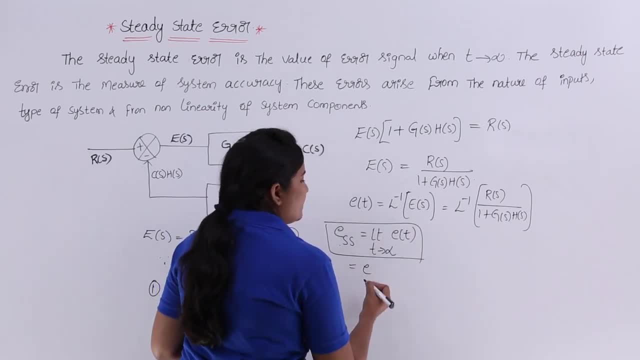 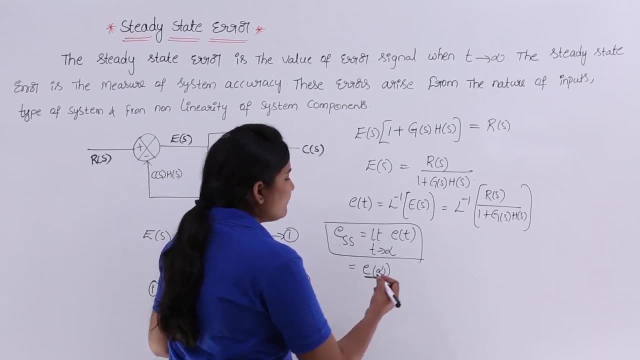 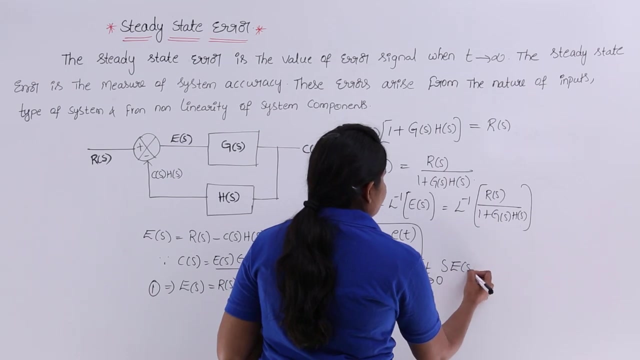 So this is nothing but limit t tending to infinity. E of t is nothing but E of infinity. E of infinity is nothing but final value of the signal. how will get final value of the signal? limit s tends to 0, S into E of S. So according to final value theorem, we: 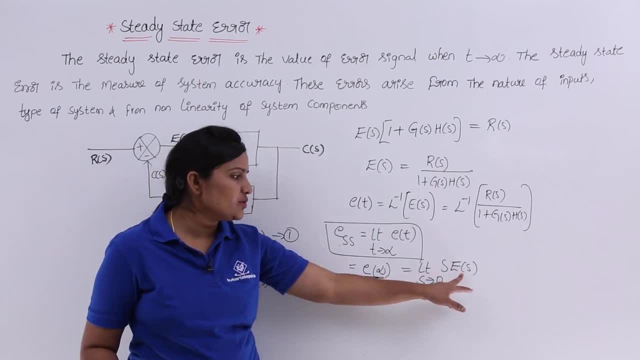 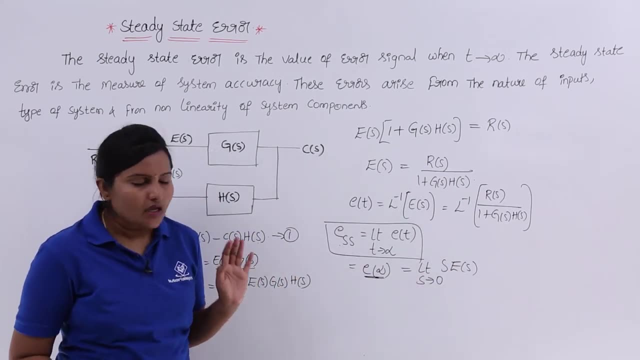 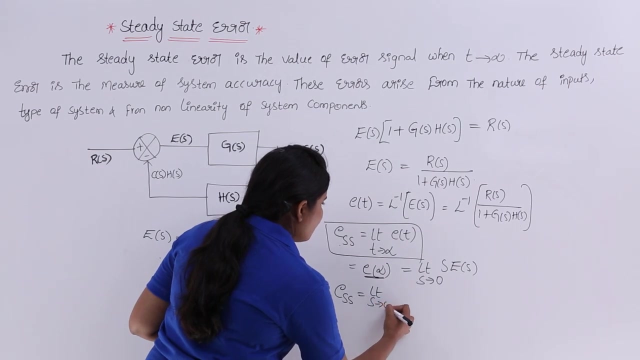 can write: E of infinity is equivalent to limit s tends to 0 S into E of S. So this we written accordingly to final value theorem. Now, from now onwards, we can write this steady state error, as limit s tends to 0 s into E of s. We can write like this or like this: this according to final. 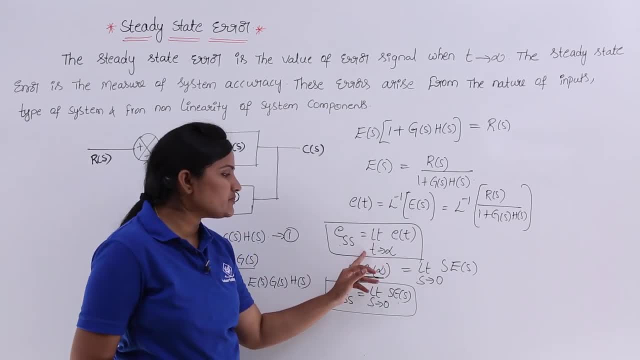 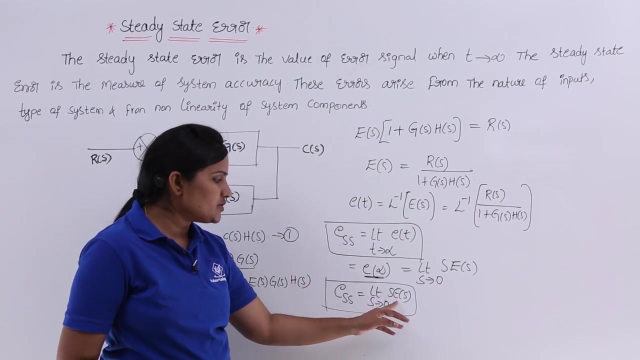 value theorem. So if they given E of t, simply by substituting t tending to infinity, you can get steady state error. If you are given with E of s, then just by taking final value of that E of s, final value of that error, transform, that means limit s, tends to 0 s.